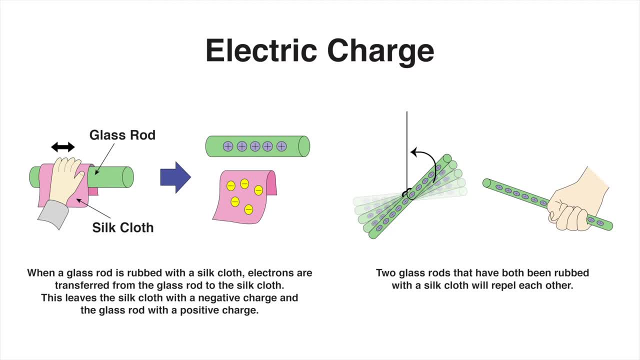 If you then hang up that glass rod, you'll see that the glass rod will leave the glass rod with a positive charge. You can bring another glass rod which, as you can see in this diagram, when you bring the two rods together they'll actually repel each other. So another demonstration that charge. 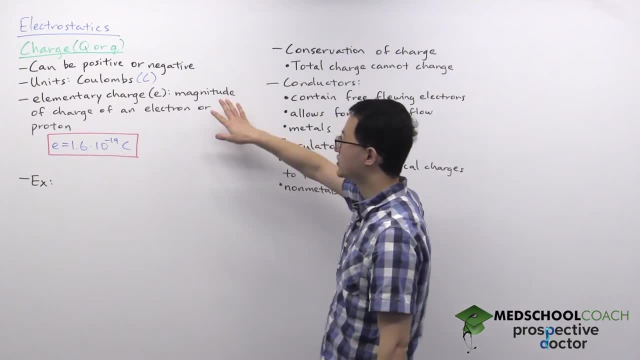 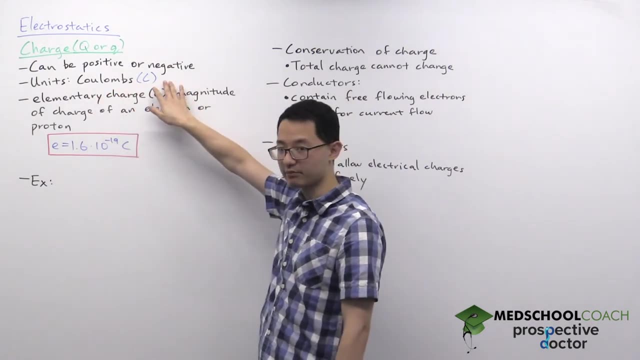 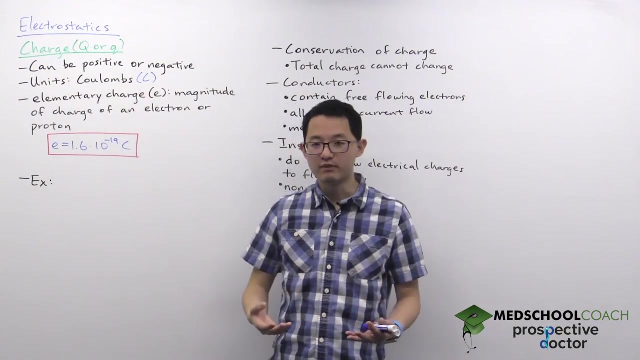 exists, All right. so charge can be both positive or negative. The units that we have for charge are coulombs, which is denoted by capital C. This is another one of the basic SI units. Now, in terms of how much charge comes from, they come from atoms, And within atoms there are electrons and protons. 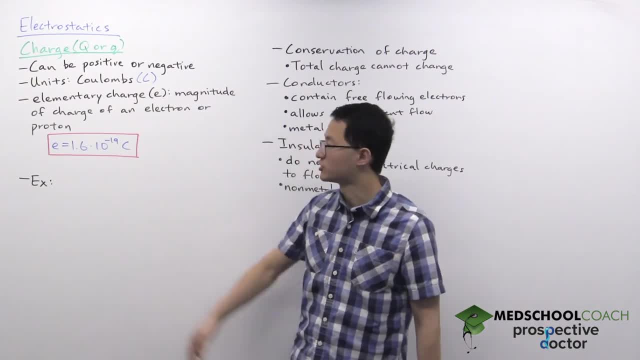 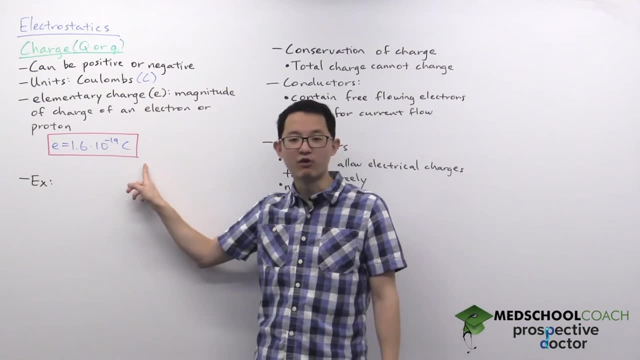 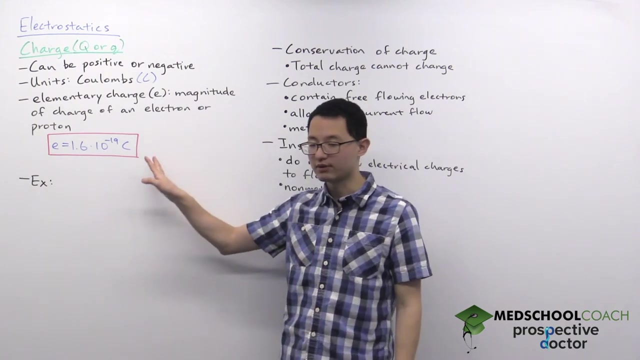 Electrons and protons have the same magnitude of charge, which we call the elementary charge. The elementary charge is denoted by lowercase e and it's equal to 1.6 times 10, to the negative 19 coulombs. So that means a proton has a charge of plus e and an electron has a charge of minus e. 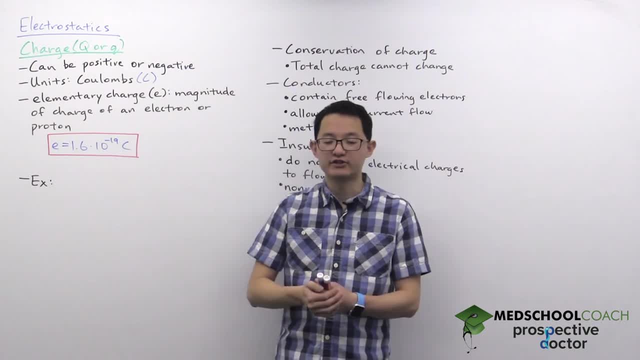 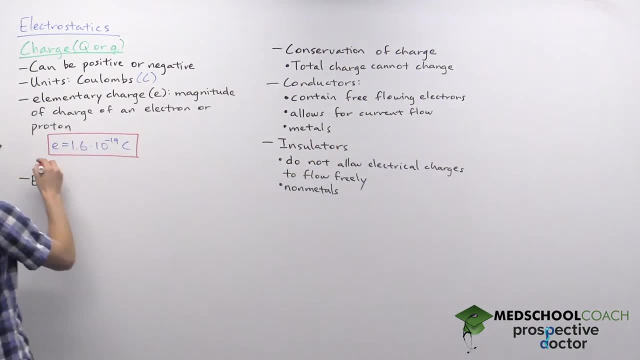 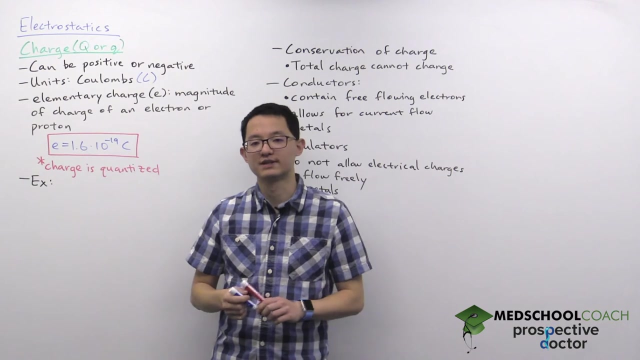 And since when you're transferring charge you can only transfer them in with electrons or protons, we can say that charge is quantized. They're always transferred in increments of e. So, for instance, we can consider a few examples. Let's say we're looking at a chloride anion. 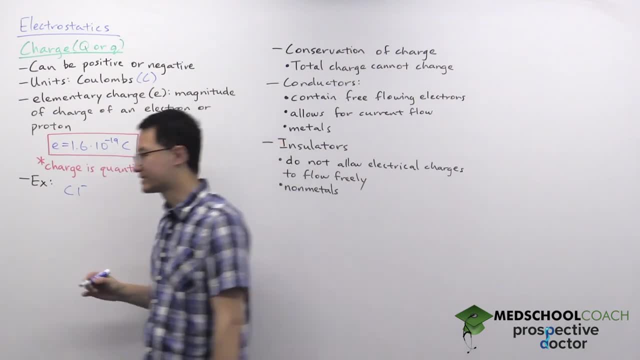 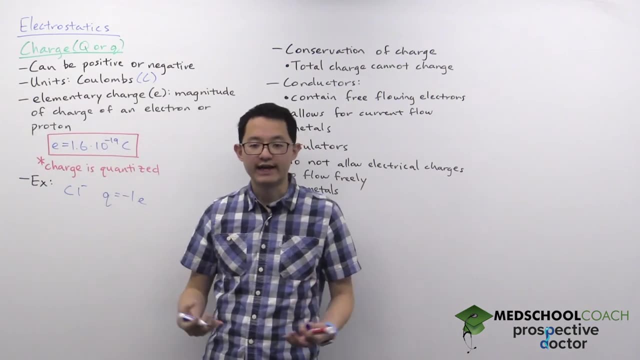 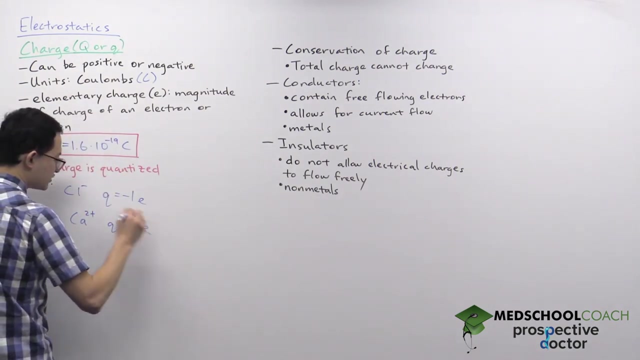 Well, if we're looking at a chloride anion, we're looking at a chloride anion and we're looking at a chloride anion. If we were to take a look at another ion, for instance a calcium cation, we would say that it has a charge of plus 2e. 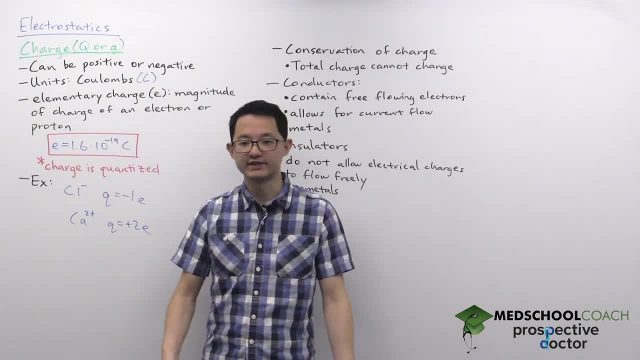 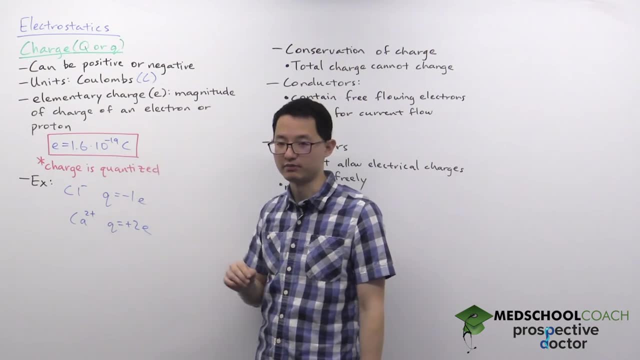 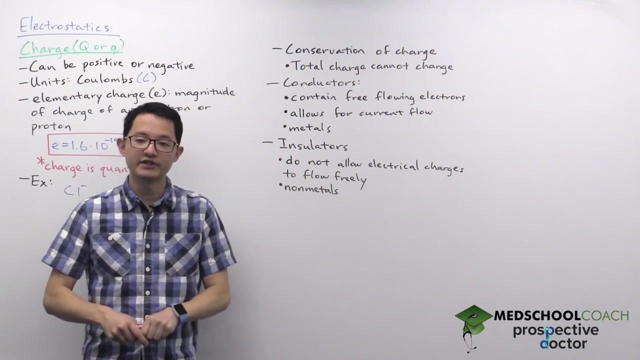 So the charge that any atom or object has is always some integer multiple of e, the smallest quantity of charge possible. Okay, So the next thing I want to talk about is conservation of charge. Conservation of charge is fairly straightforward and essentially says total charge cannot change. 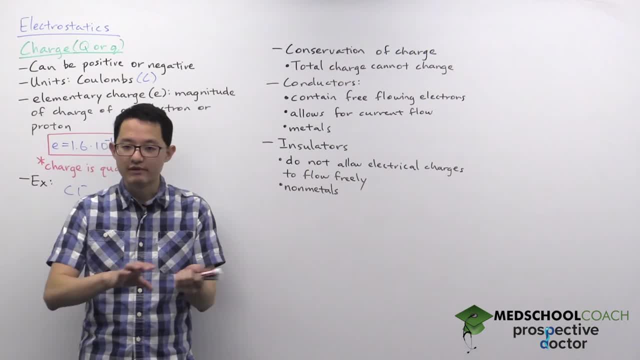 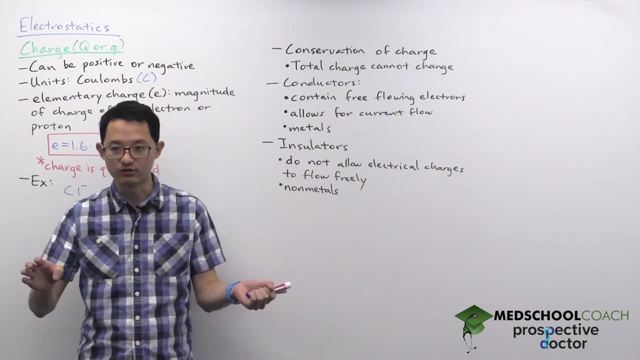 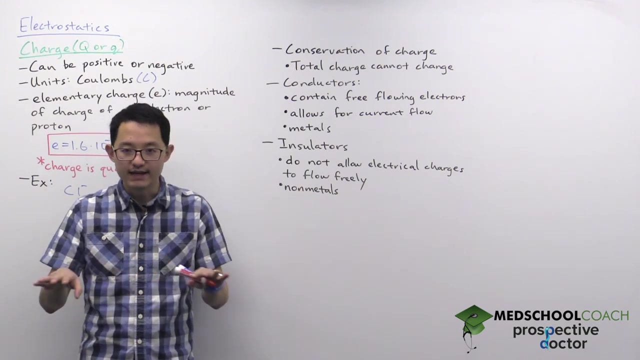 So, for instance, when you take a glass rod and you rub it with silk, the glass rod takes on a positive charge and that's because the electrons were transferred to the silk. So even though the glass rod lost charge, the silk gained that charge. so there was a net no change in the total charge.